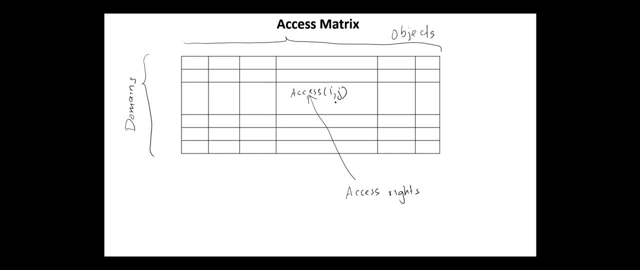 The entry Axis IJ defines the set of operations that a process executing in domain DI can invoke an object OJ. The Axis Matrix can implement policy decisions concerning protection. The policy decisions involve which rights should be included. Usually, the user decides the contents of the Axis Matrix entries. 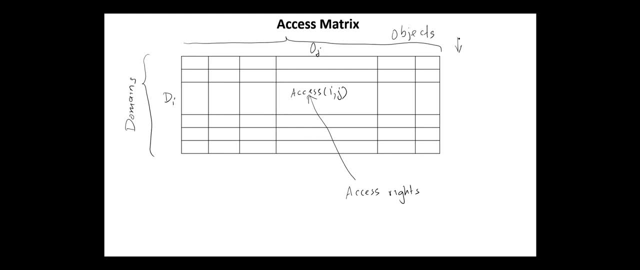 When a user creates a new object, the column of that object is added to the Axis Matrix with the appropriate initialization entries. as decided by the creator, We may include some rights in some entries in this new column and other rights in other entries, as required. 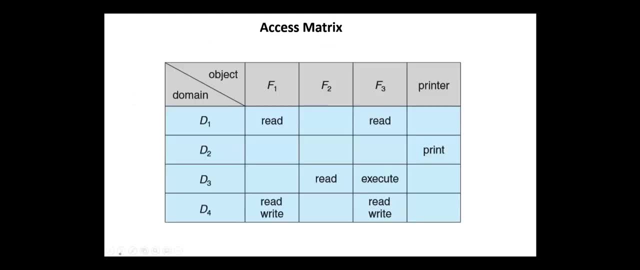 Consider the following actions. To create a new object stated an array would not hold an action to be indicated in the Hised Mhm of if this user adjusts this object or if no object relieve and into는 this object in the created member, We may include some rights in terms ofطwe can call this file Fandu. 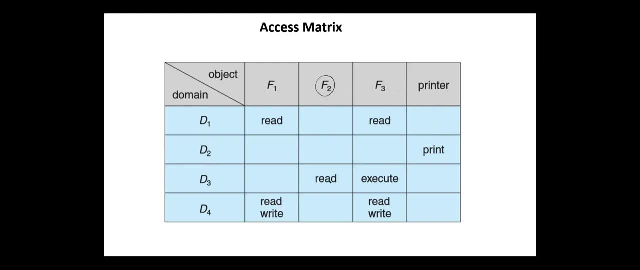 Let us consider the following Axis Matrix with four domains and for objects: A Process Executing in domain One can read files F1 and F3, A Process Executing in domain Two can use the laser printer. And a process executing in domain 3 can read vivat 2 and execute file. 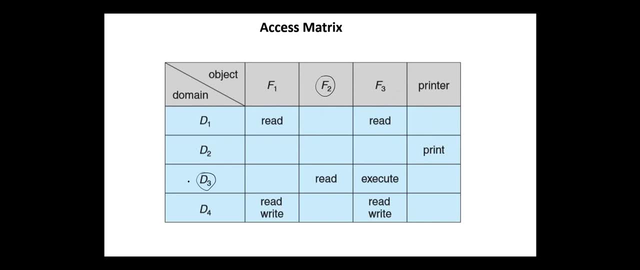 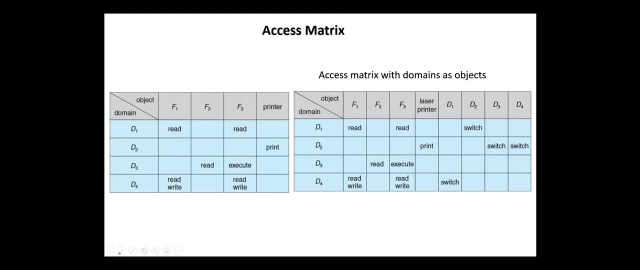 3, etc. executing in domain 3 and the laser printer can be used only by a process executing in domain 2. the axis matrix provides a mechanism for defining and implementing strict control for both static and dynamic association between processes and domains. the switch operation can be used to switch from: 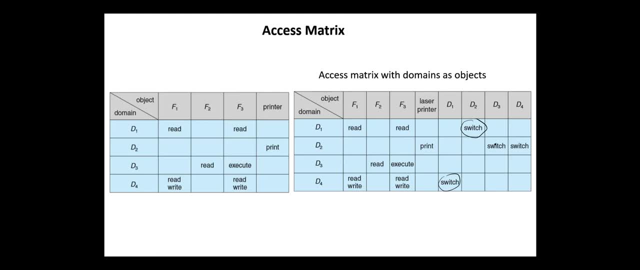 domain to another domain switching can be controlled by including domains among the objects of the axis matrix. switching from domain di to domain DJ is allowed if, and only if, the axis right switch belongs to access IJ. for example, in this figure, domain, one can switch only to domain to. 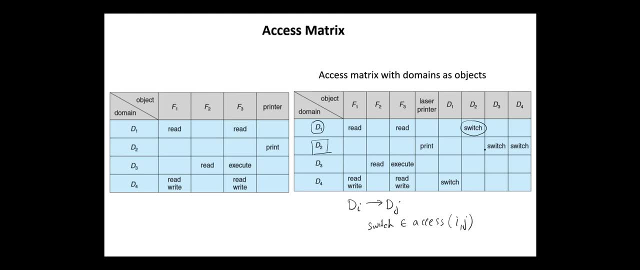 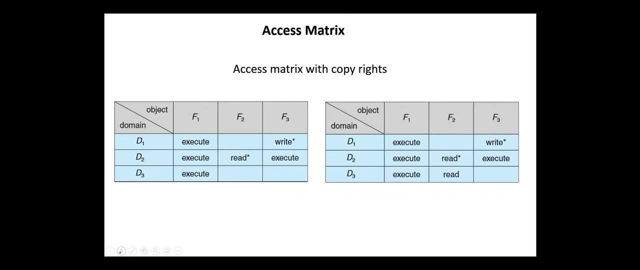 you. domain two can switch to both domains d3 and default, and domain default can switch only to domain d1. allowing control changed in the contents of the axis matrix entries requires three additional operations: copy, owner and control. The ability to create an access write from one domain or row of the axis matrix. 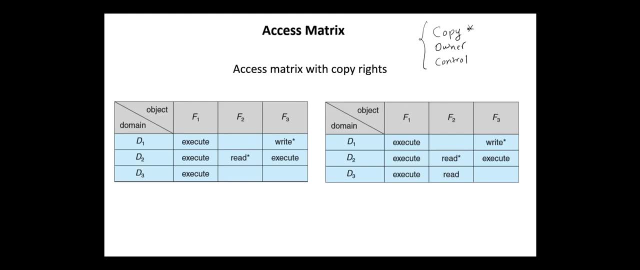 to another is denoted by anesthetic append to the access rite. the copyright allows the access right to be copied only within the same column for which direct is defined. For example, in this figure, a process executing in domain 2 can copy the read operation in to an entry associated with the slightly less than root or one questions section. 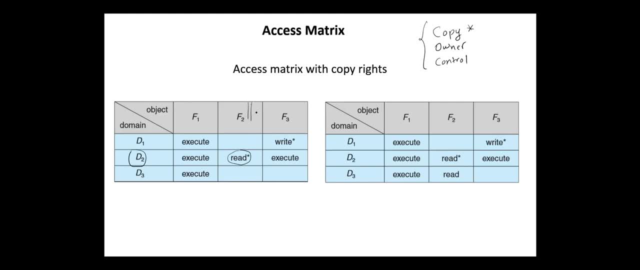 copy of this เง IJ 2 is successfully interpreted in domain 2. should you enjoy this vision into any entry associated with the file F2. as shown here, Propagation of the copyright may be limited. This means when the right R asterisk is copied. 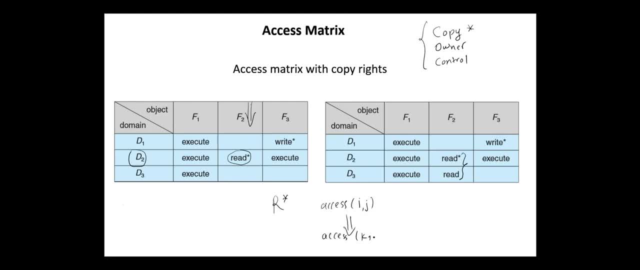 from axis IJ to axis KJ, only the right R is created, So a process executing in domain DK cannot perform the copy on the right R. Another variation is used when a right is copied from axis IJ to axis KJ. it's then removed. 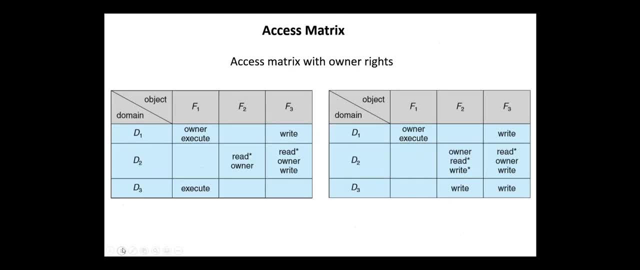 from axis IJ, The additional removal of new rights is performed using the owner right. If axis IJ includes the owner right, then a process executing in domain DI can add, access And remove any right in any entry in column J, For example, in this figure: 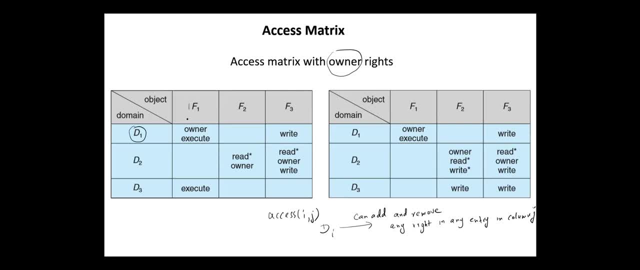 domain D1 is the owner of the file F1. Therefore it can add and delete any valid rights in column F1. Here the right execute in domain D3 is removed In the same manner. domain 2 is the owner of file F2..